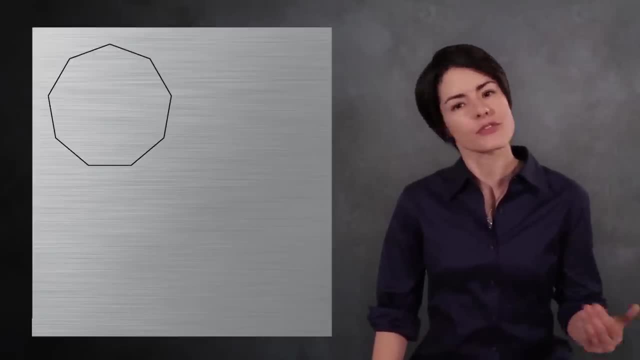 If the polygon has n sides, then there are n different reflections. When the polygon has an odd number of sides, the axes of symmetry are the lines through the vertices. 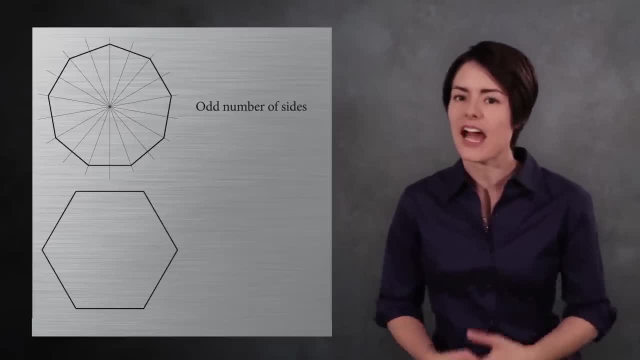 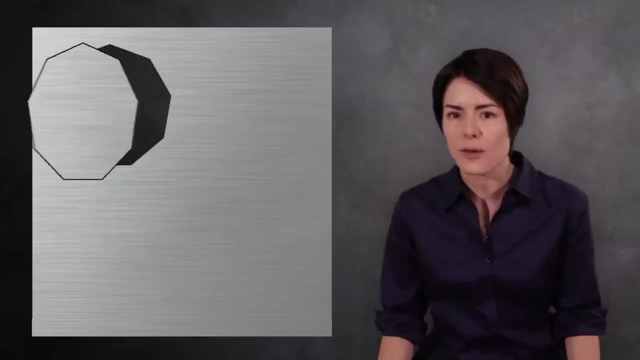 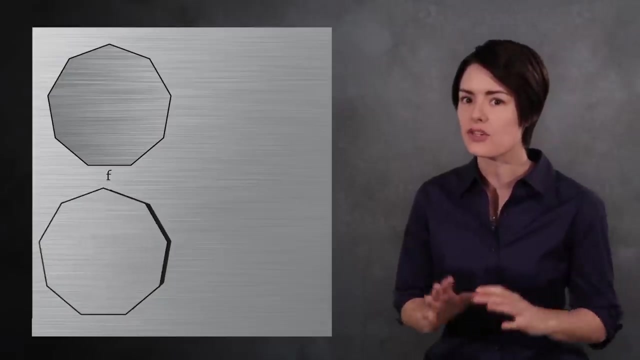 If there are an even number of sides, then the axes of symmetry are the lines through opposing vertices and the lines through opposing sides. Let's start with reflection about the vertical axis and call this transformation F for flip. If you flip twice, you return to the original position of the shape. So F squared is e. 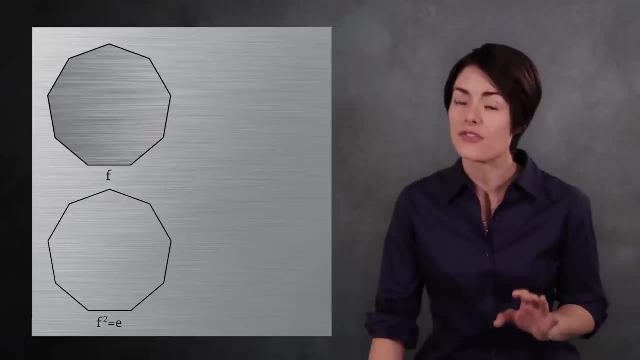 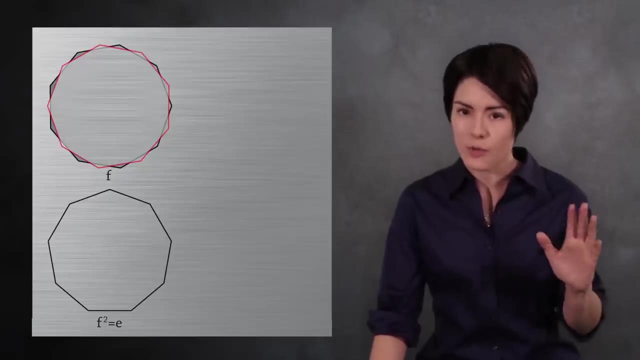 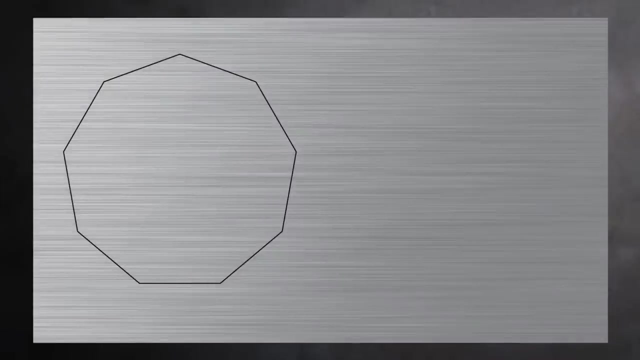 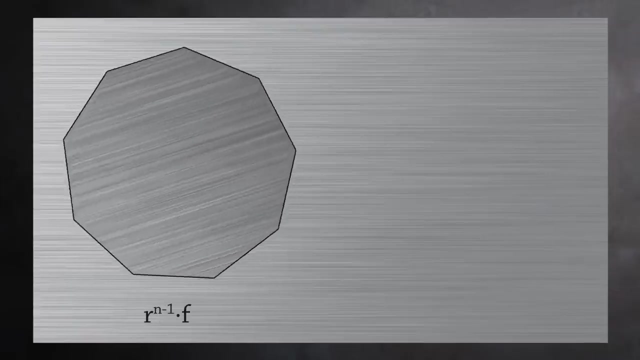 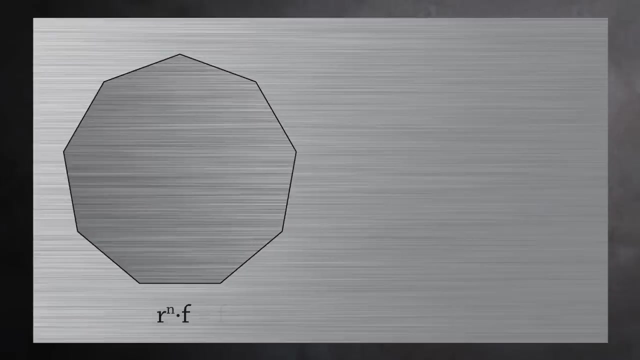 By the way, this assumes that our polygon is aligned vertically. If the polygon is slightly tilted, then a flip about the vertical axis would not tilt. The vertical axis would not be a symmetry. The before and after are different. The remaining symmetries of this shape can be found by combining R and F. If you first flip the shape, you can then perform up to n-1 rotations to get the remaining symmetries. If you perform n rotations after a flip, you get the same result as just a flip. So there are a total of 2 n different symmetries for a regular n-sided polygon. Because there are only a finite number of elements in this group, we say the dihedral group is a finite group. 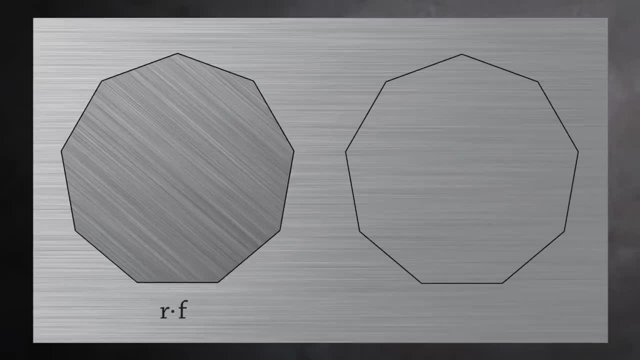 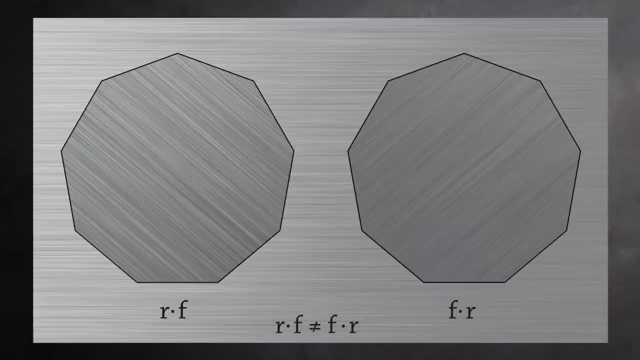 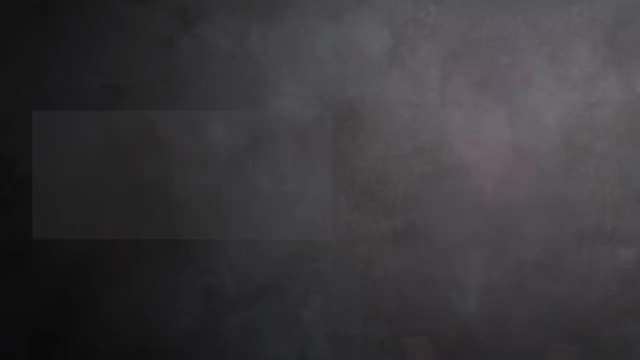 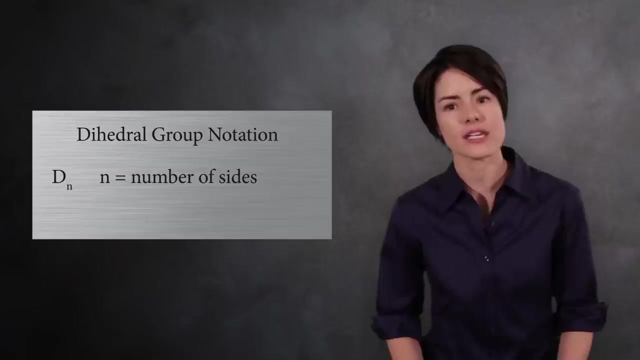 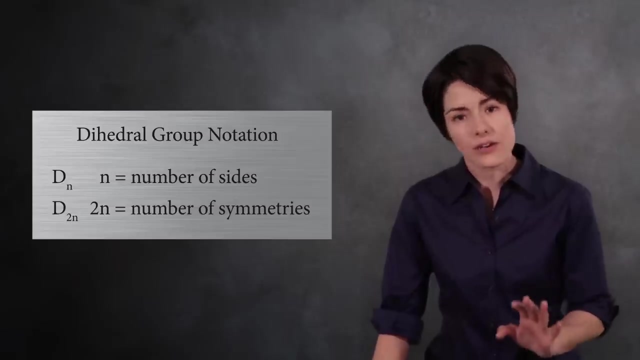 And notice that if you flip, then rotate, you get a different outcome than if you rotate, then flip. In other words, R times F does not equal F times R. The dihedral group is not commutative. Another way to say this is nonabelian. Unfortunately, there are two competing notations for the dihedral group. Some people write d sub n to indicate the number of sides of the polygon. Others write d sub 2n to highlight the number of elements in the group. So be careful, since for example, d sub 6 could either mean the dihedral group of the hexagon, or the dihedral group for an equilateral triangle. 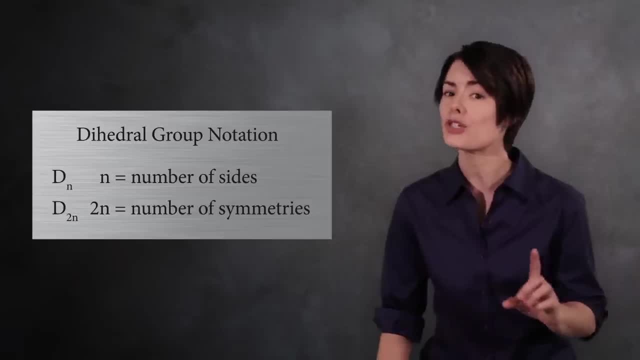 When you're talking to your friends about group theory, be sure you agree on notation. 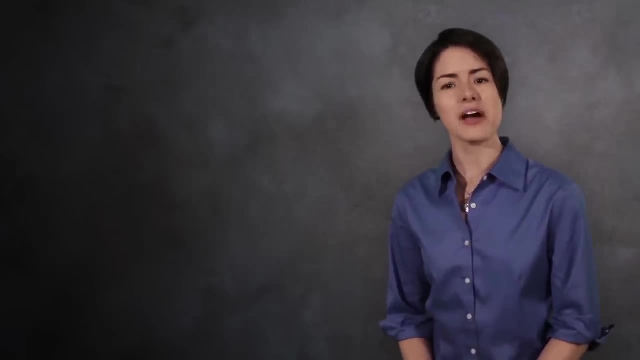 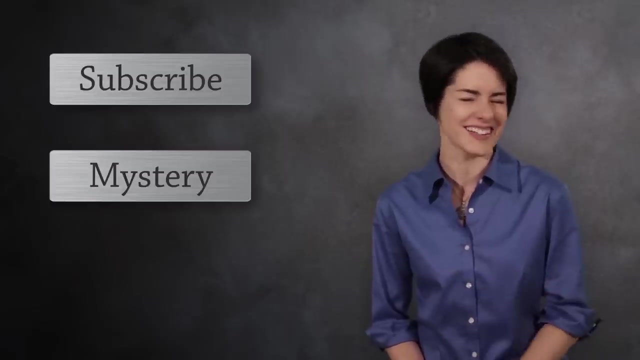 Thank you for watching to the very end of this video. You have a nice attention span! I like that in a viewer. I especially like that in a subscriber. Oh, will you look at that! Buttons! Just love to be clicked. No pressure or anything, though. I'll just give you two a moment. Okay.